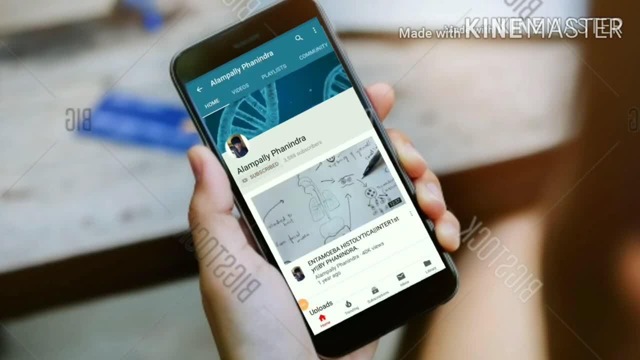 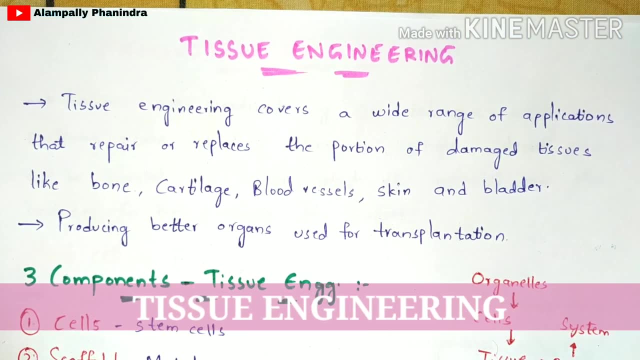 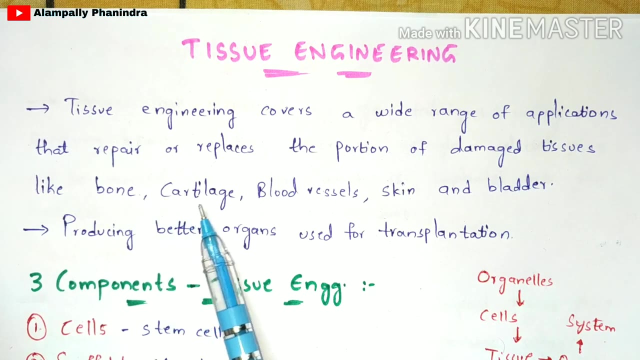 Hi friends, if you like my videos, subscribe my channel and also press the bell icon for the latest updates. So in this video let us discuss about tissue engineering. Tissue engineering covers a wide range of applications that repair or replaces the portion of damaged tissues like bones, cartilage, blood vessels, skin and bladder. 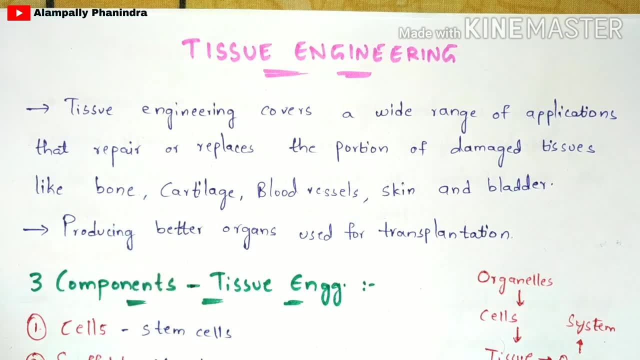 And in this video I'm going to explain you in the case of a bone. So, for example, damaged tissues are nothing, but this bone is considered as a tissue right And once that bone got fractured then you will consult into the hospital. 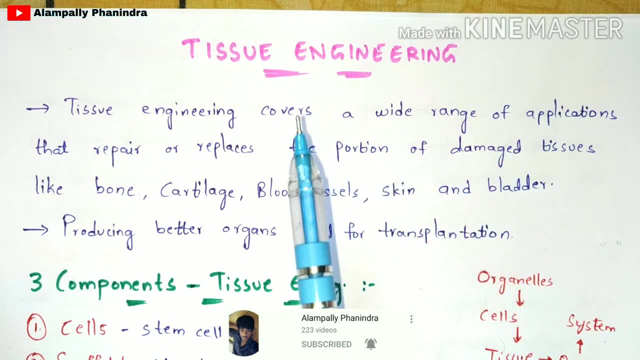 And once you consult the hospital then the doctor will do this tissue engineering technique on that particular damaged tissue in such a way that that bone which has been fractured will be recovered right, So that recovering of that bone from the fracture, from the damaged position is called as a tissue engineering right. 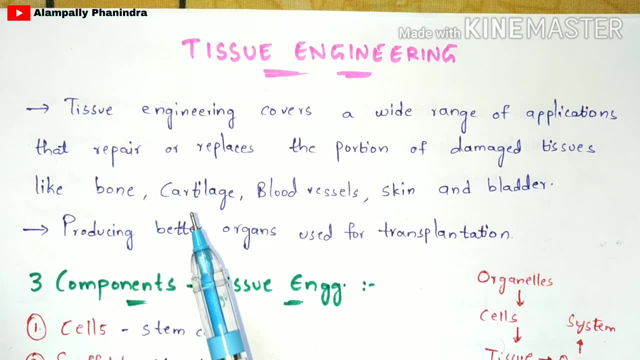 And not only the bone. this tissue engineering is also applied for the tissues like cartilage, blood vessels, skin, as well as the bladder. right And now, this tissue engineering. the main goal of this tissue engineering is to develop and to construct the transplantable tissue and to also to produce the better organs for the transplantation. 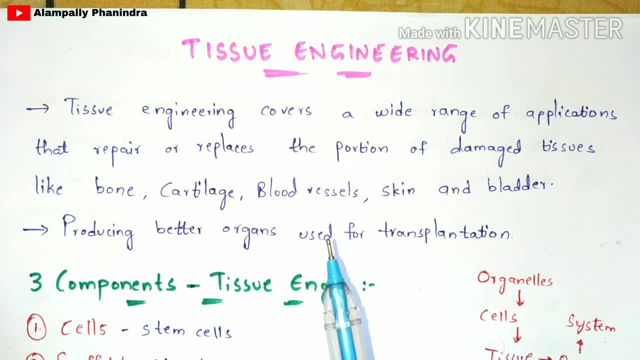 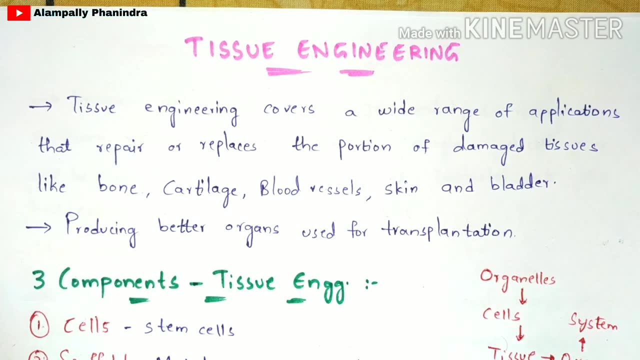 So how this tissue engineering technique is performed. What is the protocol which is present behind this tissue engineering? Each and everything will be explained in detail in this video. So what are the three major components which are mainly used for this tissue engineering? First is cells. 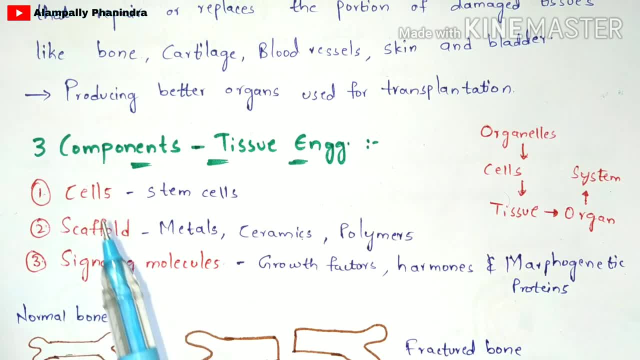 Second scaffold And the third is signaling molecules. And what does this cells mean? Cells includes stem cells. So what are the stem cells? Stem cells, we know that the stem cells are of two types: adult stem cells as well as the embryonic stem cells. 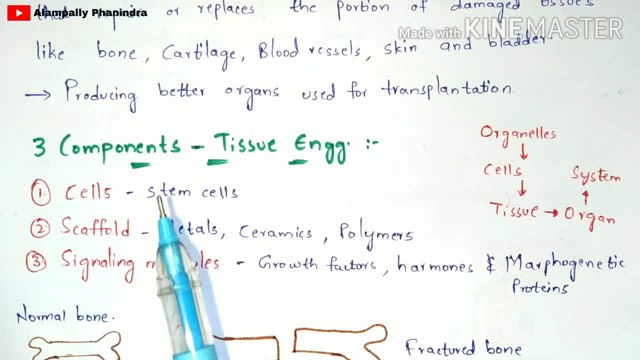 But in the case of this tissue engineering, most widely used stem cells are adult stem cells. So why not embryonic stem cells? Why only the adult stem cells? Because adult stem cells has only the capacity to develop the tissue into a new form. okay, 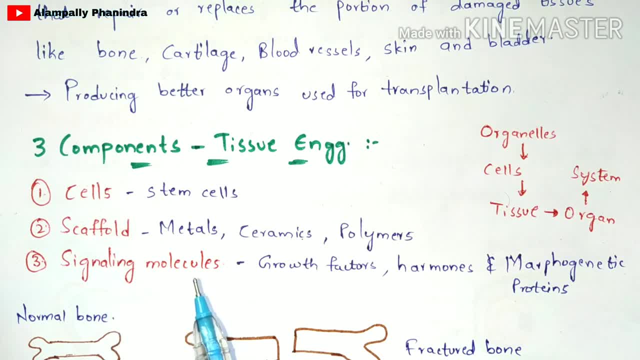 It will develop the new tissue. Only the adult stem cells has the capacity when compared to that of embryonic stem cells. So adult stem cells are highly preferred for this tissue engineering technique. And these adult stem cells are very, very few, and even the cell division process will also be done very, very slow, and even what happens is that only few cells will be formed even when it undergoes the process of the cell division. okay, 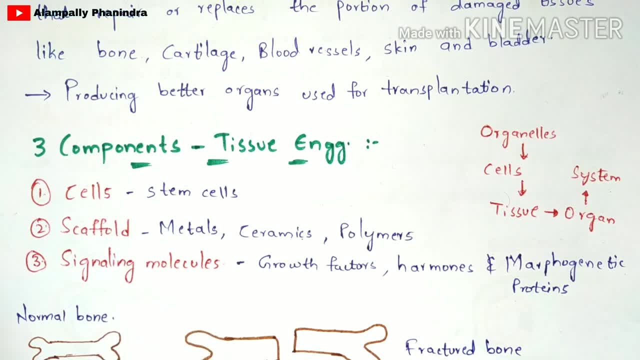 And now coming to the scaffold. Scaffold is used for the growth and development of the cells. The scaffolds are used for the growth and development of the cells And it also provides the mechanical strength to the cells And it also provides the mechanical strength to the cells. 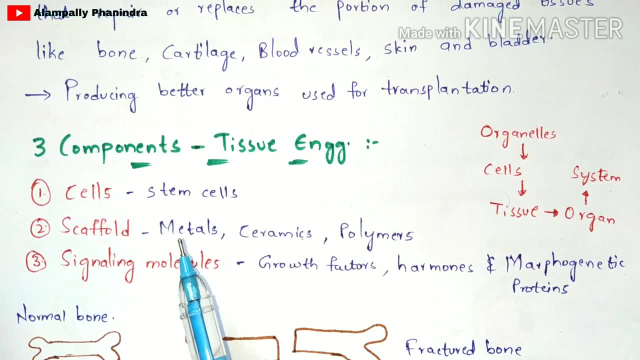 Right. Majorly used scaffolds are like what we say synthetic and synthetic. what is a synthetic natural scaffold like, for example, if you take metals, ceramics and polymers? So all of these are nothing but the synthetic natural scaffolds. So these are mainly used for the development and also for the and also providing the mechanical strength for the cells. 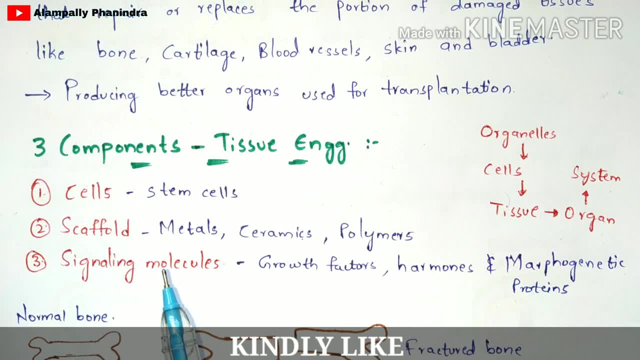 And now coming to the third one: signaling molecules. So what are the signaling molecules? basically, Signaling molecules are nothing but the bioactive molecules or biomolecules. So what are the signaling molecules? basically molecules like growth factors, hormones and morphogenetic proteins. So all of these both. 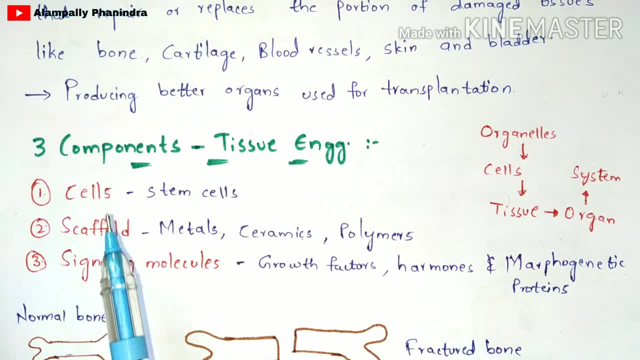 scaffold as the signaling molecules will act as a nutrient medium for the cells. So once the cells will be composed with this scaffold as well as the signaling molecules, then the cells undergoes a proliferation, and once the proliferation will be done, then it will get divided rapidly, right? 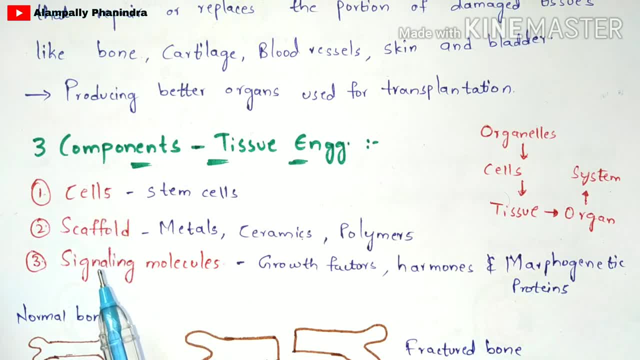 So this acts like a nutrient medium. This scaffold, as well as the signaling molecules, will act like a nutrient medium for the cells to get divided, to get proliferated. So this is about the components which are mainly required for the tissue engineering and before entering into the 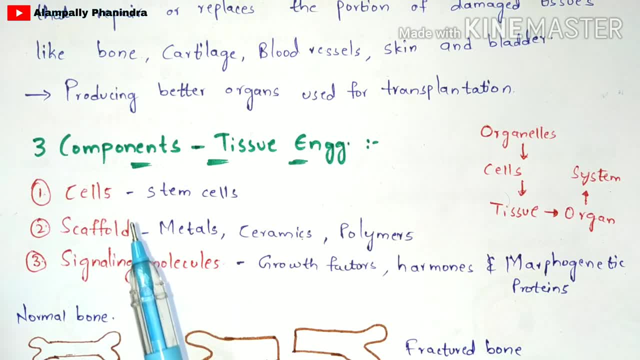 procedure of this tissue engineering, one of the most important thing I wanted to say. So what is that? is from the junior classes we are learning that. So what is that? organellist will form the cells and the cells will form the tissues, and the tissues forms organs, and the organ will form the. 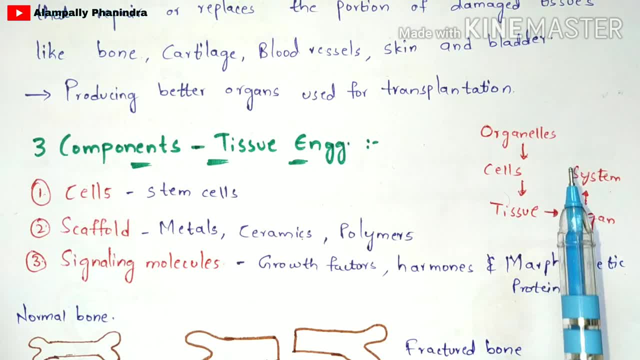 total organ system, where how the human body will be designed. So this is how the human body will be designed and this is how the human body is formed actually, from which the organellist will form the cells and cells will form the tissue. So in this video, you should remember, in this topic of the tissue, 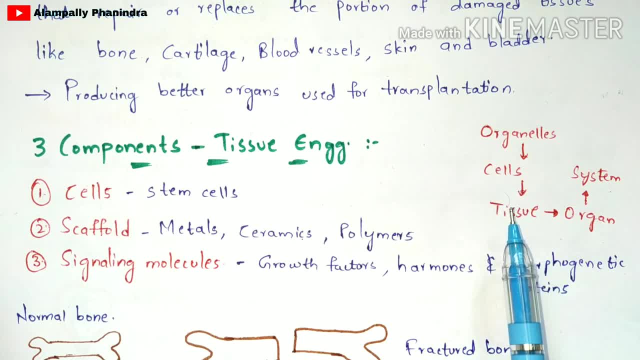 engineering. you should remember that the cells will form the tissue right. So why this is needed in this procedure of the tissue engineering? I am going to explain it later. So firstly let us discuss about that procedure of this tissue engineering. So in the first step, what you are 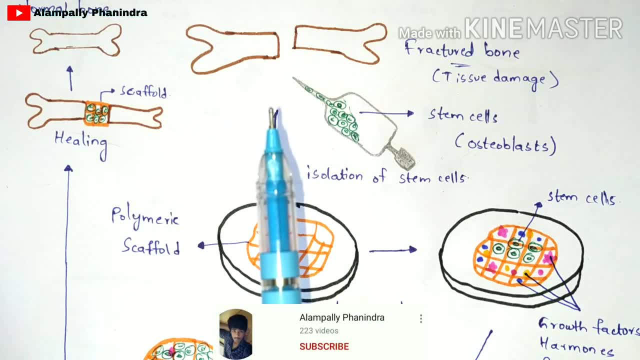 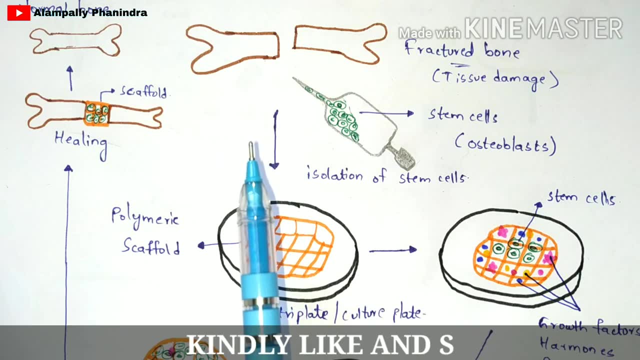 going to do is that you are going to select a patient. So what type of patient you are going to select, I have said you before itself. In this case, I am going to take a bone, a damaged tissue called as a bone, right. So we are going. 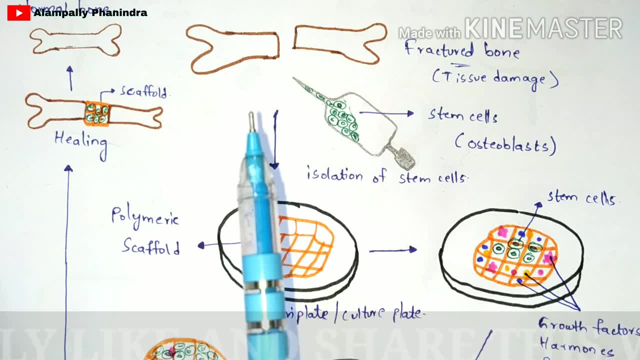 to select a patient and make sure that the patient bone got fractured, So say, this is a bone which has been got fractured and this bone, this is a bone of that particular patient whose bone got fractured and this is called as a tissue damage. This is called as a tissue damage because the 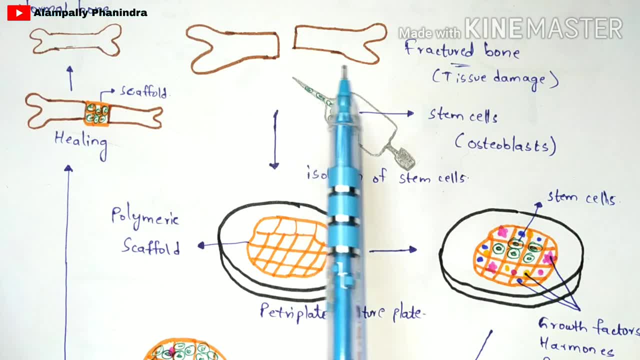 bone is nothing but the tissue. As it got fractured, it is called as a damage. Hence it is called as a tissue damage. And now, from this fractured bone, what you are going to do is that you are going to isolate stem cells from that particular bone, right? So in this way we are 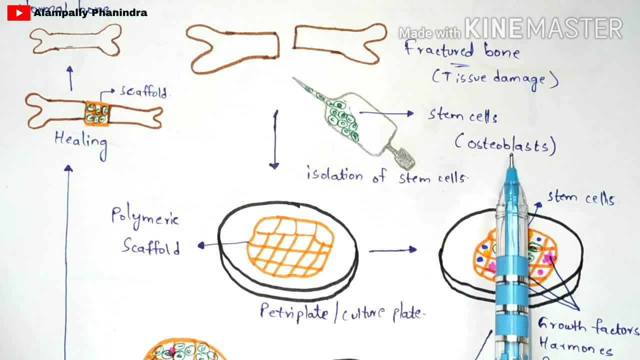 going to isolate the stem cells, And the stem cells which are going to isolate are nothing but the osteoblasts. Osteoblasts are nothing but the cells which are related to the bone are called as osteoblasts, right. So from from this particular fractured bone, you are going to isolate the 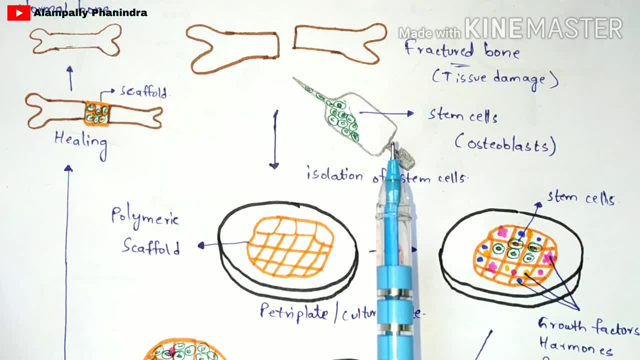 osteoblasts. So in the third step, what are you going to do Now? keep these stem cells apart, I mean, keep this osteoblasts apart, And, on the other hand, what you are going to do is that you are. 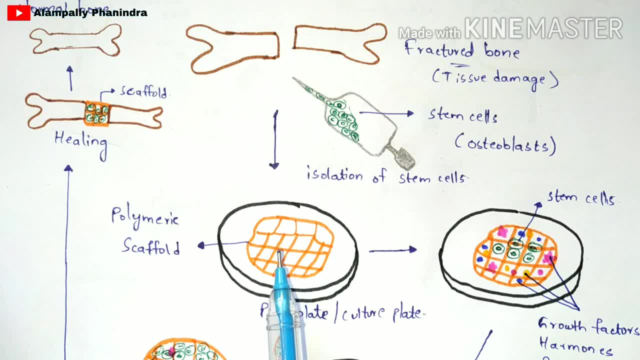 or a sculpture plate, or a petri dish, whatever you want to say. so on this petri plate, you are going to place polymeric scaffold. polymeric scaffold- so what i have said you in this, three components of the tissue engineering scaffold- is nothing, but it is mainly used for the growth and development of 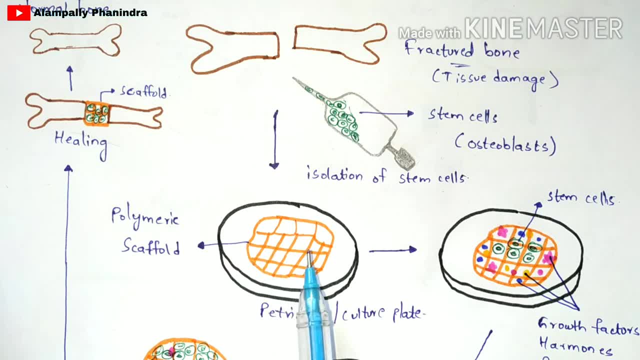 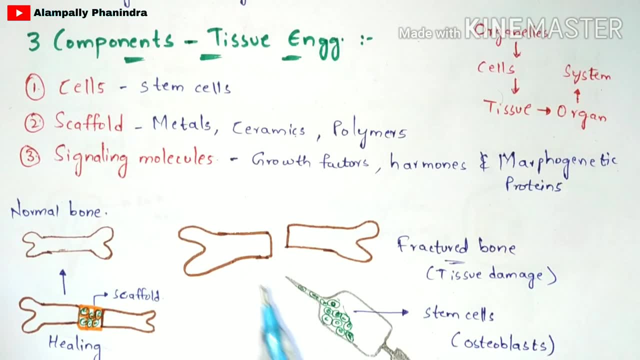 the cells and also provides the mechanical strength for the cells, right? so firstly, you are going to take a petri plate and you are going to place this polymeric scaffold- polymeric scaffold, so if you see here in the components of this tissue engineering, so what are the synthetic 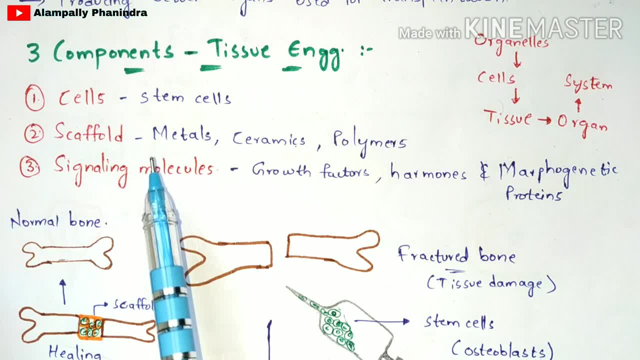 what? what are the synthetic type of? what are the synthetic type of natural scaffolds which have been used like metals, ceramics and polymers. right, and mostly preferred are polymers. so that's only the reason i have mentioned here polymeric scaffold. so this is your polymeric scaffold and 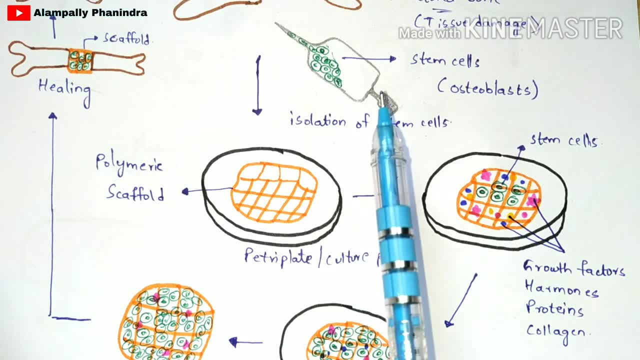 to this polymeric scaffold. what you are going to do is that you are going to place the stem cells which has been isolated from the particular type of fractured bone right though this osteoblast. are nothing but the stem cells which will be placed on this polymeric scaffold, which is placed 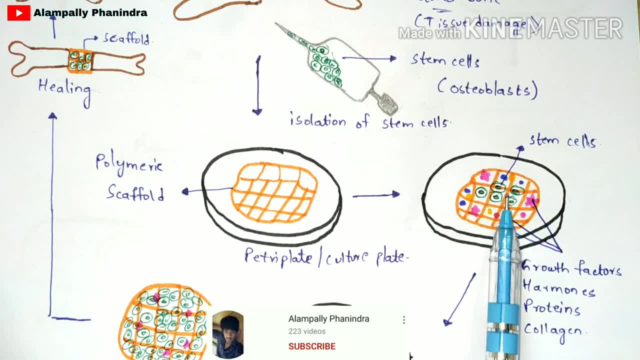 on this petri plate like this. so this green color one are nothing but the stem cells, or else this green color one is nothing but the osteoblasts. right and now to this osteoblast which is present in this polymeric scaffold, what you are going to add? you are going to add the third components. 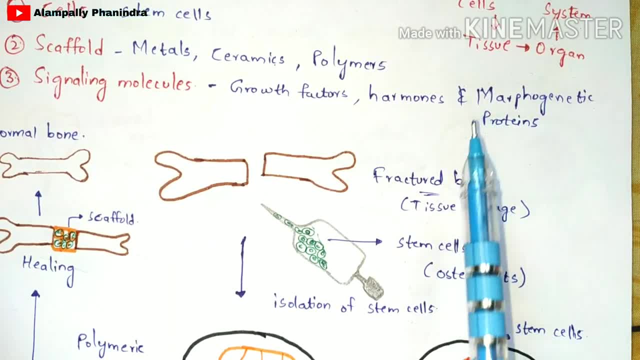 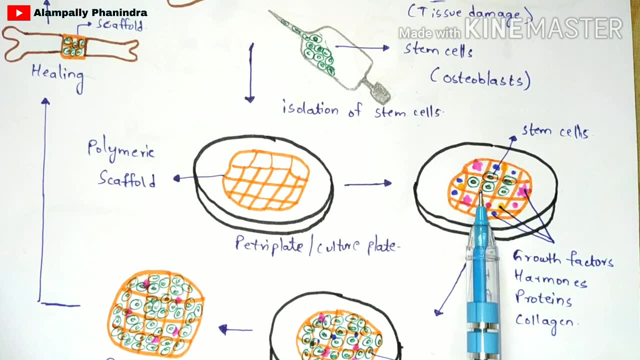 which are called as signaling molecules. so growth factors, hormones and morphogenetic factors, and even the collagen fibers, will also be added to this particular type of what we say, this polymeric scaffold, which consists of this osteoblasts. right and now what happens? and in the next step, 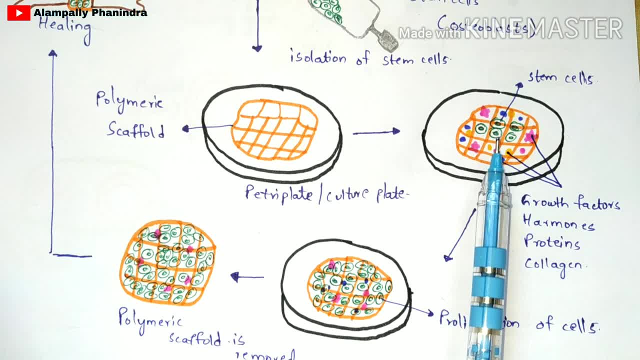 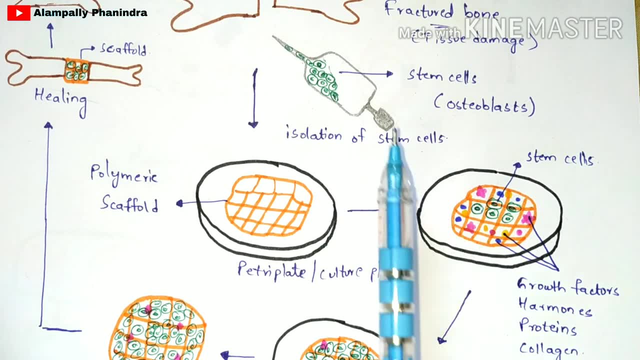 what happens is that the cells are present in small quantity, right? so here normally a large quantity of stem cells will be isolated, but here only small quantity will be added, because you are going to select a particular type of cells which are highly active, and that highly active stem cells will be placed in this polymeric scaffold which is present. 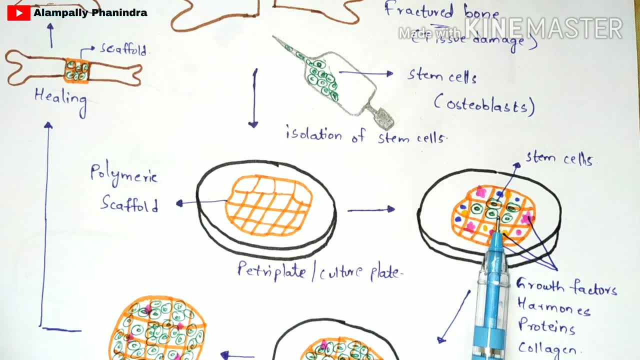 in this petri plate. and now to this petri plate, you are going to add this signaling molecules. all of these signaling molecules, this pink color one, yellow color one and as well as this blue color one, are nothing but the signaling molecules, the growth factors, hormones and morphogenetic proteins. so all of this will be added to this. and now what? 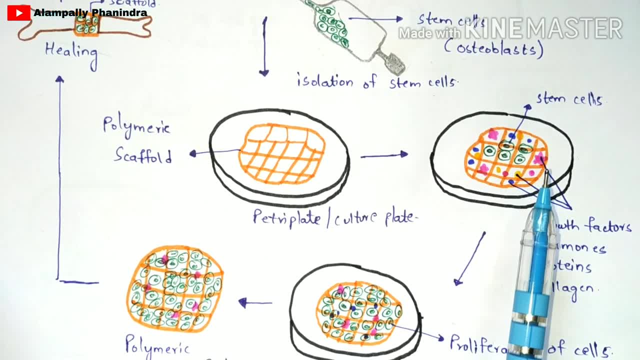 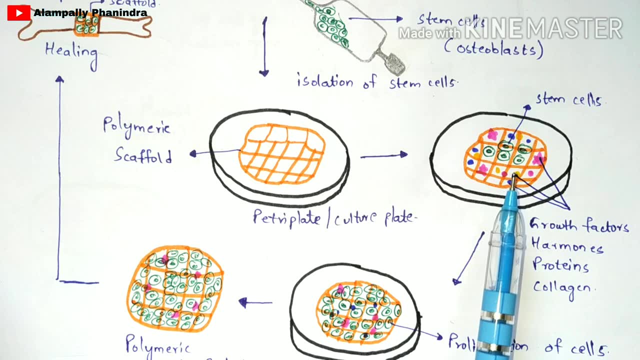 happens is that I have said you at the beginning of the video itself. so this scaffold, as well as the signaling molecules, will act as a nutrient medium for the cells. so how it acts as a nutrient medium for the cells in such a way that that cells will use as that particular nutrient. 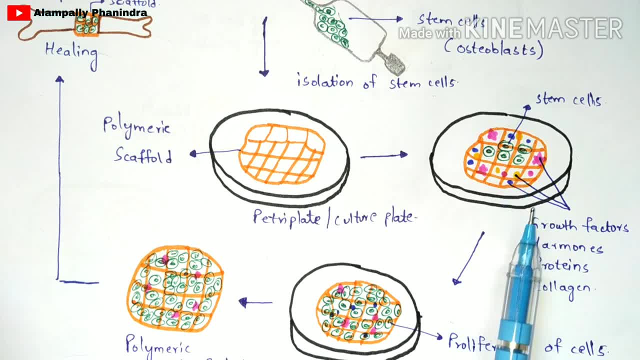 medium. the nutrients is present on this scaffold as well, as the nutrients is present in this in the form of these growth factors. all of this will be utilized by the stem cells and once it get utilized, Then proliferation- the stem cells will undergo proliferation. so how the 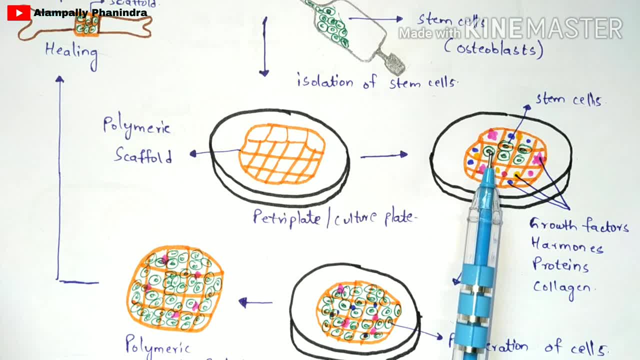 proliferation occurs. what is mean by proliferation? proliferation is nothing but the process which undergoes the cell division, rapid cell division. so the number of the cells, the number of the stem cells, has been increased because of the proliferation of the cells. so how it got increased? because the nutrient 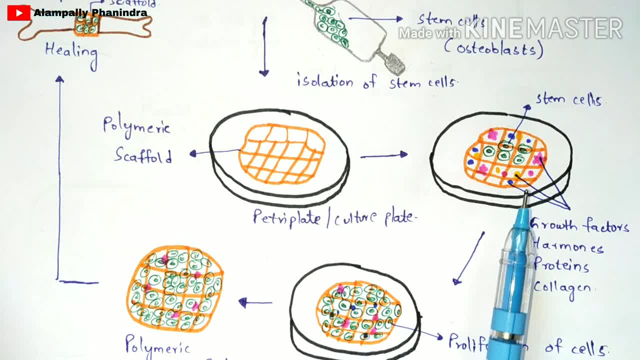 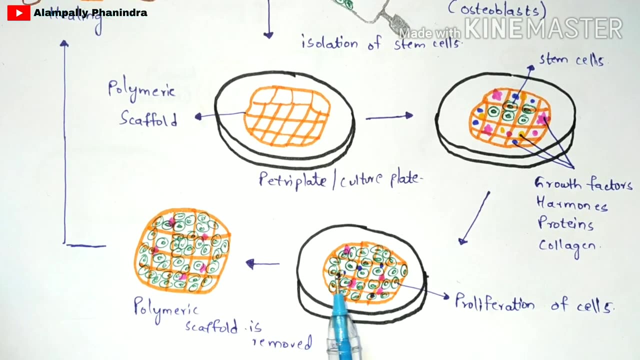 medium is present. it utilizes that nutrient medium in such a way that that stem cells will gain energy from the nutrient medium and it will get proliferated. it will get cell division process occurs in the stem cells and the number of the quantity of that cells will be increased right and now in the 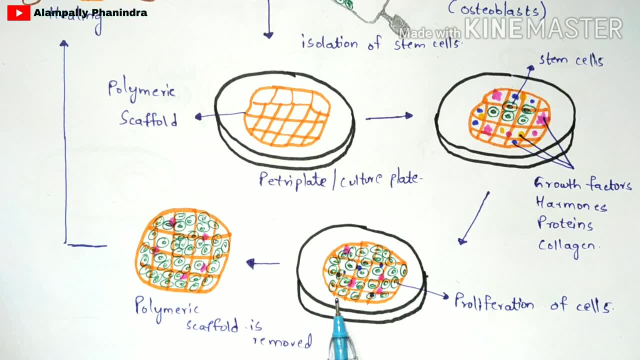 next step. what you are going to do is that you are going to remove this polymerous scaffold which is present in this petri plate and make sure that the polymerous scaffold consists of the stem cells right, and here the quantity of the growth factors, hormones, proteins, collagen- has been decreased. why? because 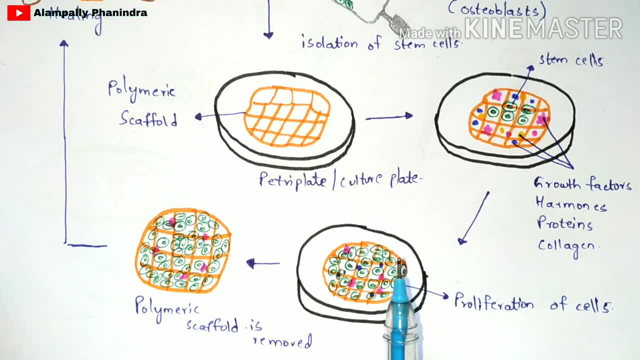 this stem cells utilized all of these nutrients for the growth factors, and the growth factors of the protein collagen has been decreased because this stem cells utilized all of these nutrients for the development process. for the growth process, I mean to increase the quantity of this bacteria, of these stem cells, right. so for that process, the 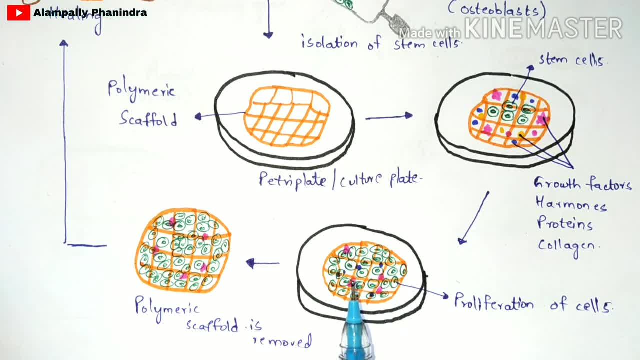 growth factors and all of the signaling molecules. quantity will get decreased because the number of the stem cells has been increased. and now you are going to remove that particular type of polymerous scaffold from this petri plate which consists of the stem cells. and now what you are going to do with this? 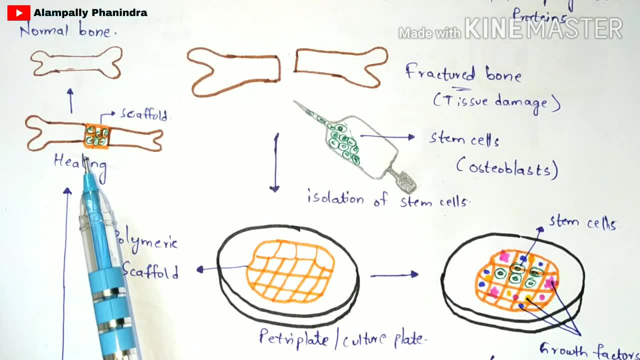 polymerous scaffold. now you are going to heal that particular type of polymerous scaffold which consists of this stem cells. right now you are going to remove this stem cells to this fractured bone. so this is a fractured bone right and at the particular place. this is a place where the bone has got fractured. 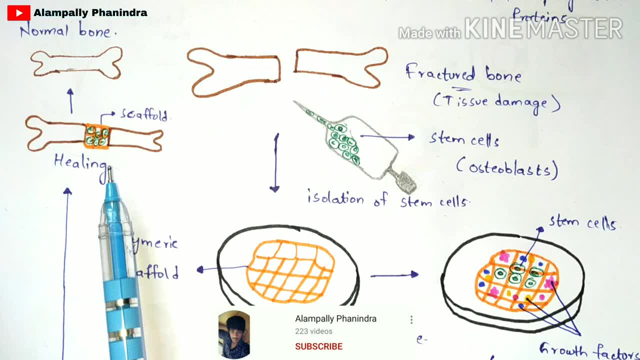 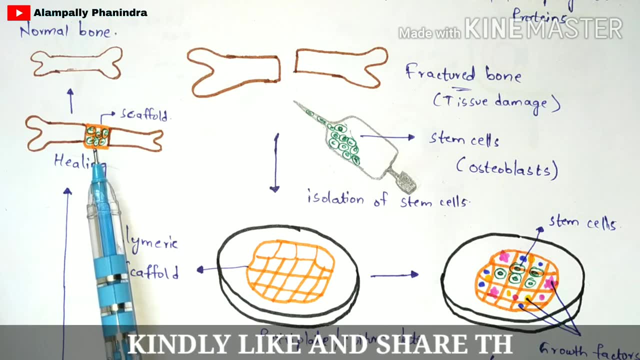 and to that place you are going to heal that polymerous scaffold which consists of the stem cells, right? so this is called a healing and within 20 days to one month, 20 days to 30 days, the this fractured bone will get converted into a normal bone. so this is how the healing occurs. this is how the normal, what we 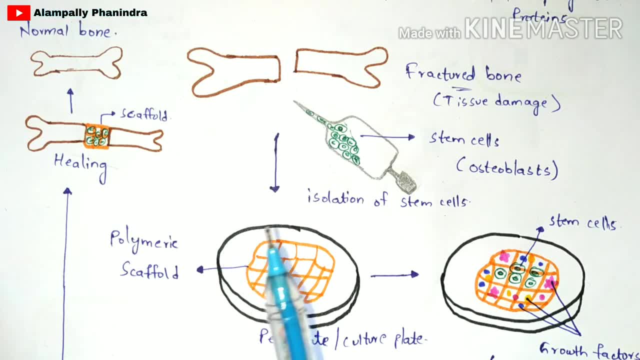 say, repairing of the tissues occurs by applying the tissue injection. so this is applying the tissue engineering process. so this is a process, whole process, which occurs in the hospital, which will be conducted by the doctors, to undergo the process of tissue engineering to convert this fractured bone into a normal bone. 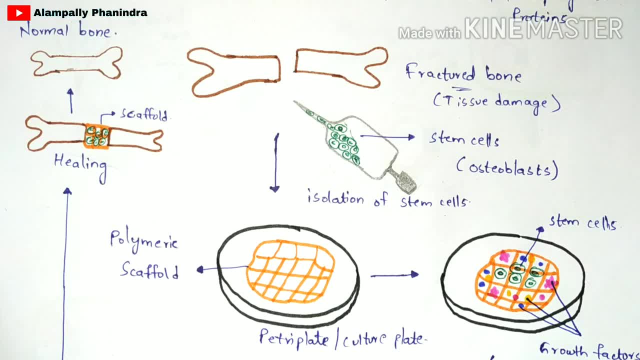 back again. so this is a process which has been done in this tissue engineering and hope you would like this video. and the notes for this topic will be given in the whatsapp group and the invite link of that whatsapp group will be given in the description box. so by using that link you can join us in the whatsapp.